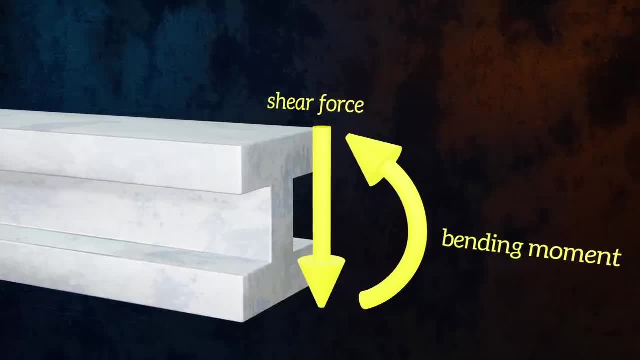 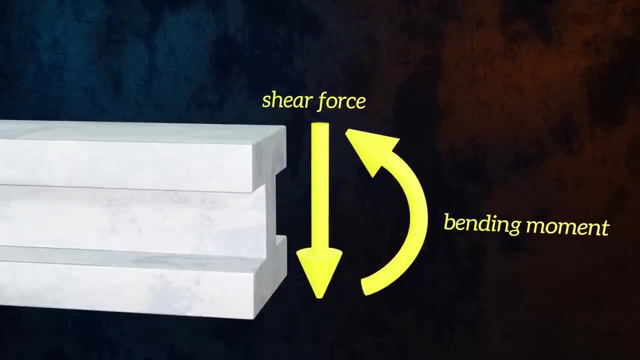 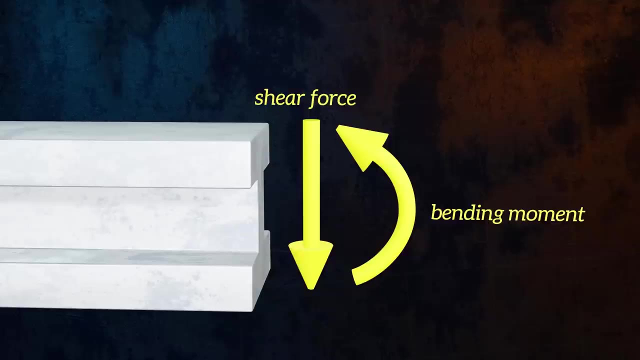 forces and one bending moment, which is a resultant of the normal internal forces. This is a very common way of representing the internal forces within a beam. Drawing the shear force and bending moment diagrams is just figuring out what these internal forces are at each location along the beam. 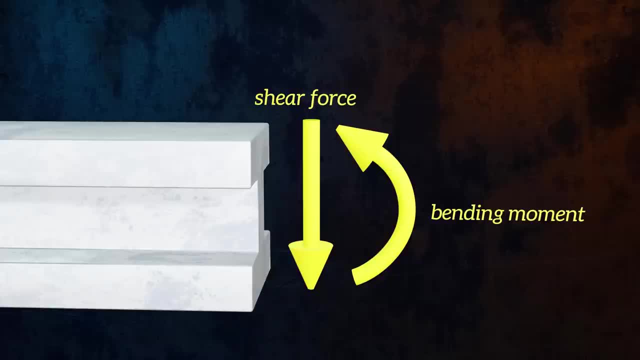 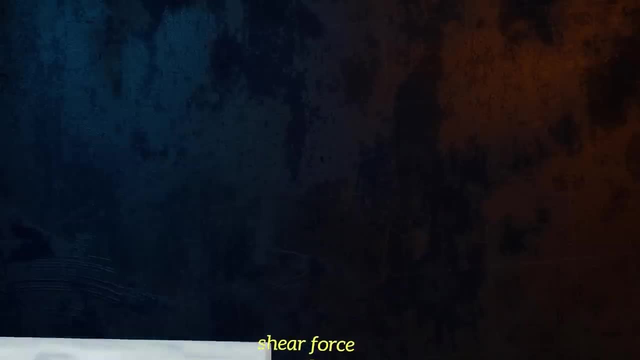 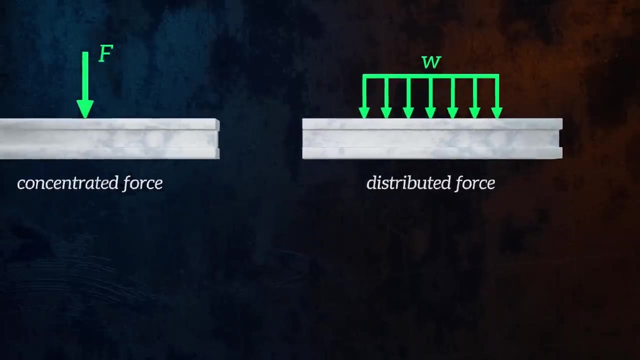 These resultant shear forces and bending moments will depend on the loads acting on the beam and the way in which the beam is supported. Beams can be loaded in a number of ways, The most common being concentrated forces, distributed forces and concentrated moments. 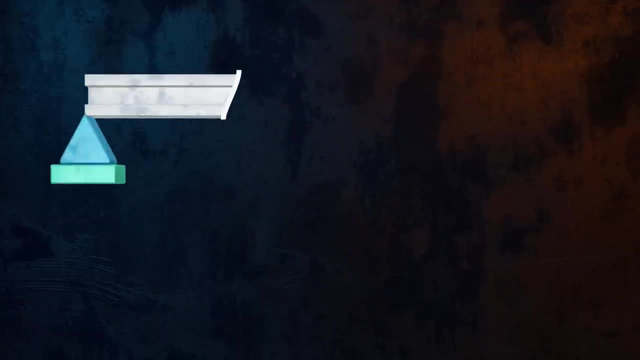 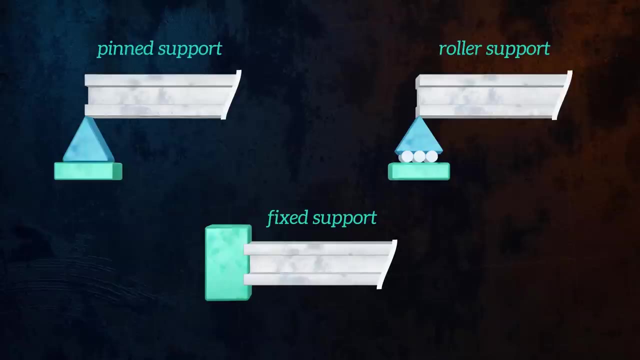 Beams can also be supported in a number of different ways. They can have pin supports, roller supports or be fully fixed, which each restrain the beam in different ways. Pin supports prevent vertical and horizontal displacements, but allow rotation. Roller supports allow rotation. 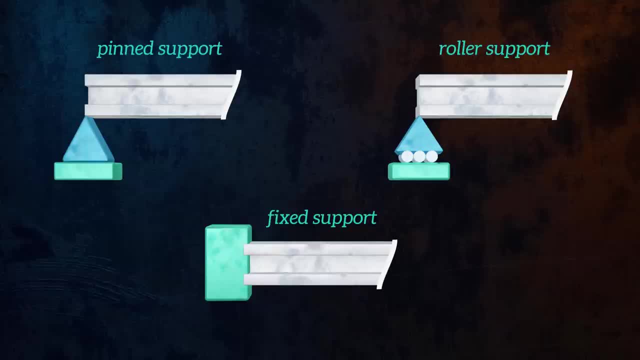 Roller supports prevent vertical displacements but allow horizontal displacement and rotation. Fixed supports prevent all displacements and rotation. If a certain degree of freedom is restrained at a support, we will have a corresponding reaction force or reaction moment at that location. For example, rotations are permitted for a pin support, so there is no reaction moment. 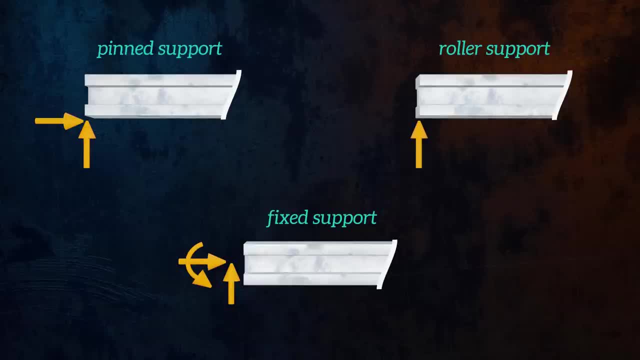 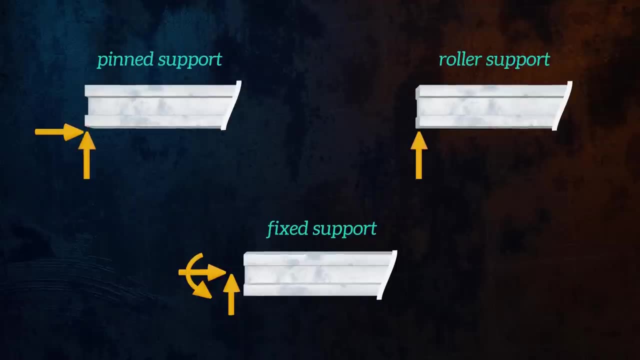 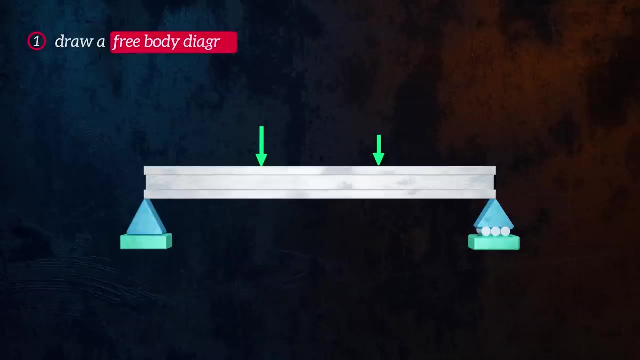 but displacements in the vertical and horizontal directions are prevented, So we will have horizontal and vertical reaction forces. So how do you determine the shear forces and bending moments within a beam? There are three main steps we need to follow. First, we draw a free-body diagram of the beam. 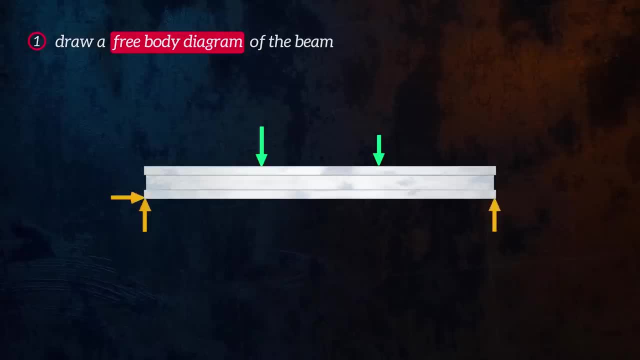 This shows all of the applied and reaction loads acting on the beam. The next step is to calculate the magnitude of the reaction forces and reaction moments at all of the beam supports. The next step is to calculate the magnitude of the reaction forces and reaction moments. 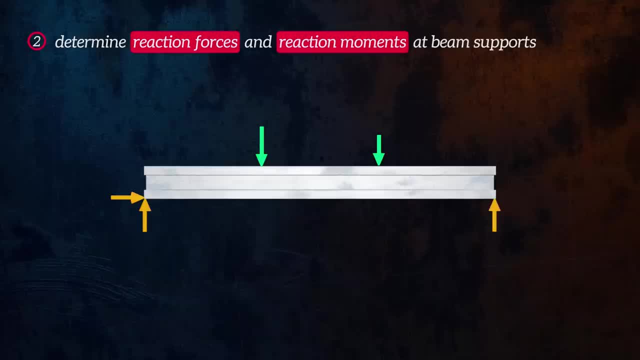 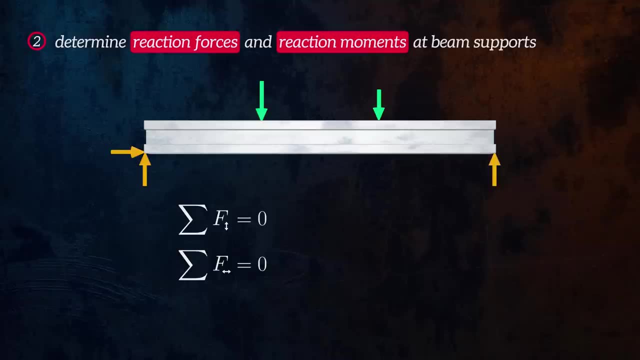 at all of the beam supports Using the concept of equilibrium To maintain equilibrium. all of the forces in the vertical and horizontal directions should cancel each other out. Similarly, all of the moments acting at every point along the beam should cancel each other out. 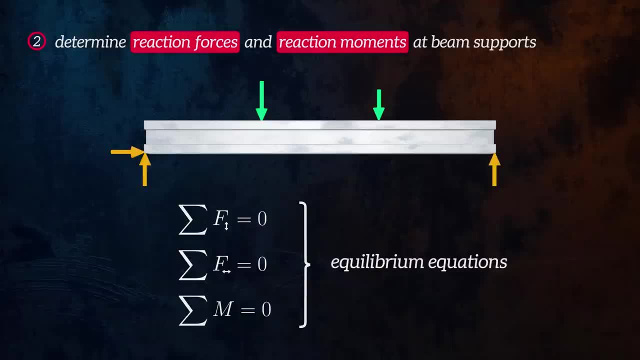 This gives us a set of simple equations we can solve to calculate the reaction forces and moments. If we can calculate all of the reaction loads using the three equilibrium equations, the beam is said to be statically determinate. For some beam configurations, like this one shown here, we won't be able to calculate. 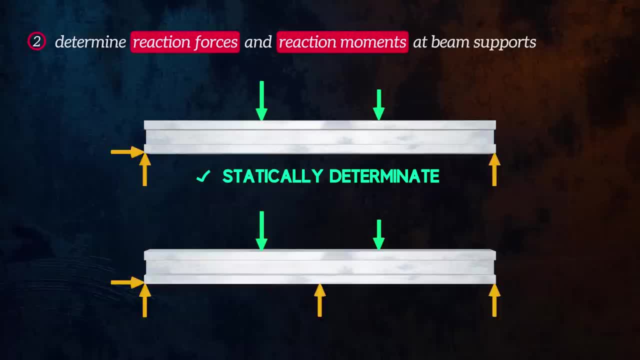 all of the reaction loads because we have too many unknowns and not enough equilibrium equations. In this case, the beam is said to be statically indeterminate. This beam has four reaction forces, but we only have three equilibrium equations. To solve this beam we would need to use slightly more complicated methods and consider boundary. 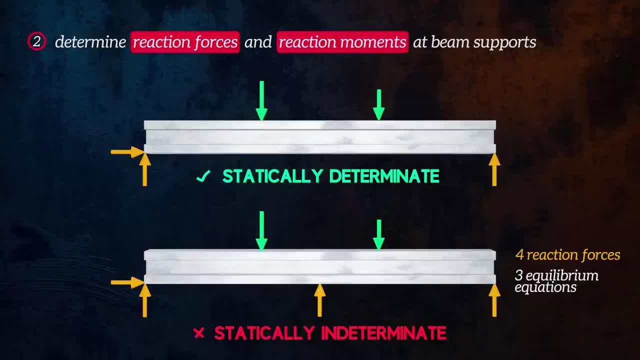 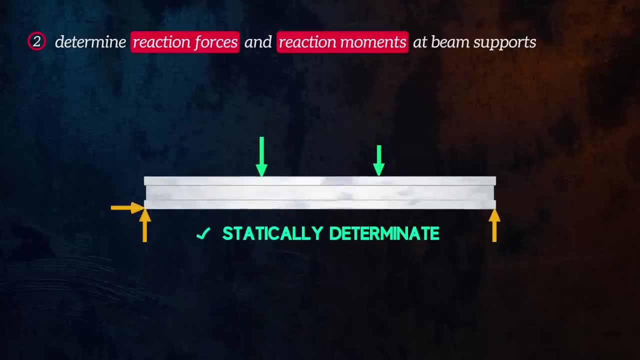 conditions. In this video, I will only cover statically determinate cases where we can use the equilibrium equations to calculate all of the reaction loads. Once we have calculated all of the reaction loads, the third and final step is to figure out the internal shear forces and bending moments at every location along the beam. 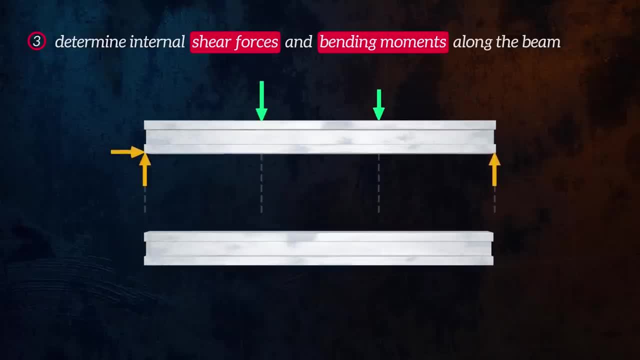 To do this, we will use the concept of equilibrium again. If we cut our beam at any location, the internal forces and moments need to cancel out the external forces and moments so that equilibrium is maintained. This allows us to easily calculate the shear force and bending moment at each location. 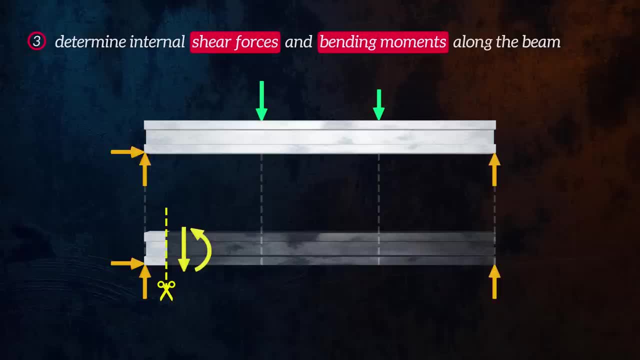 along the beam. All we need to do is start from one side of the beam and move the location of the cut along the beam, calculating the shear forces and bending moments as we go. Now is a good time to define the sign convention we will be using. 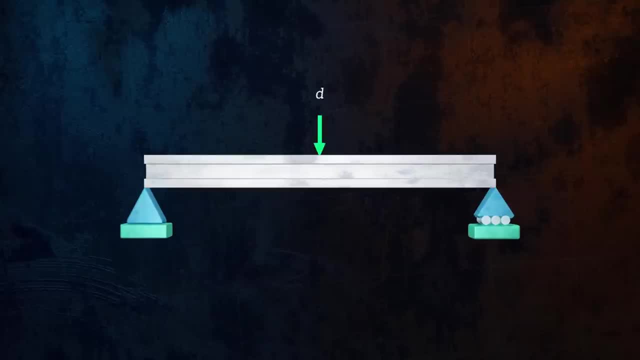 Let's start with the sign convention. Apply forces will be positive if they are acting in the downwards direction. For shear forces and bending moments, the positive sign convention will be, as shown here, If the beam is on the left side of our cut, shear forces pointing downwards will be positive. 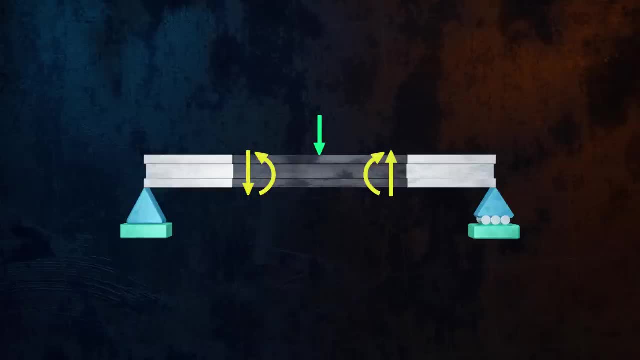 If the beam is on the right side of our cut, shear forces pointing upwards will be positive. Positive bending moments will be those that put the lower section of the beam into tension. Another way to think about it is that bending moments which cause sagging of the beam are 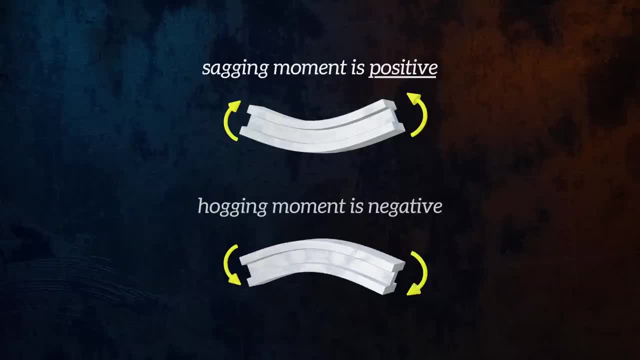 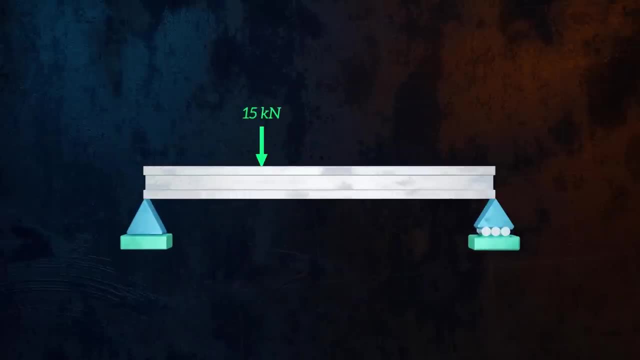 positive and those that cause hogging of the beam are negative. Let's take a look at an example of a beam with pinned and roller supports loaded by two concentrated forces. First we draw the free-body diagram. We can then use the equilibrium equations to determine the unknown reaction forces at 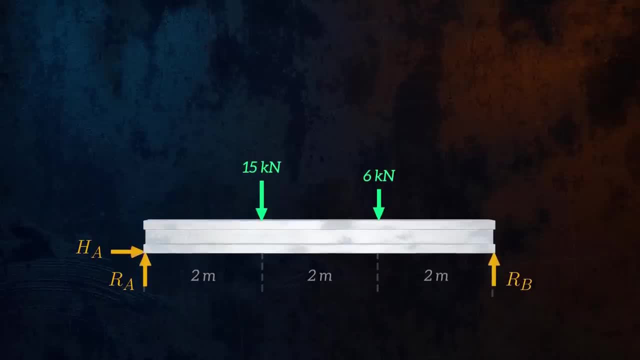 point A and point B, The sum of the forces in the vertical direction is equal to zero. so rA plus rB is equal to 15 plus 6.. Because hA is the only horizontal force, it must be equal to zero. 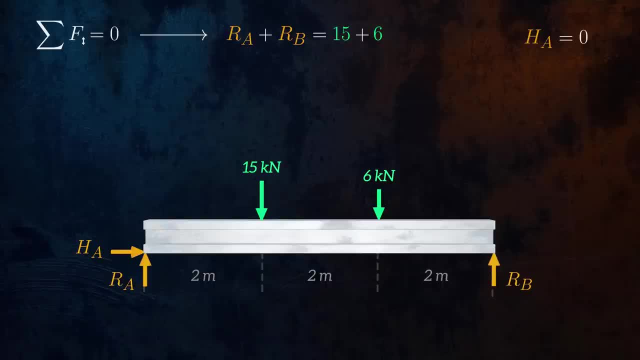 We also know that the sum of the moments about any point along our beam must be zero. Let's consider the moments about point B. That gives us this equation, which we can solve to determine that rA is equal to 12.. By substituting rA into the previous equation, we can deduce that rB is equal to 9.. 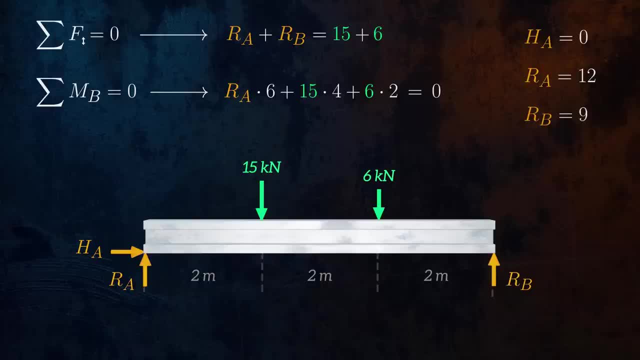 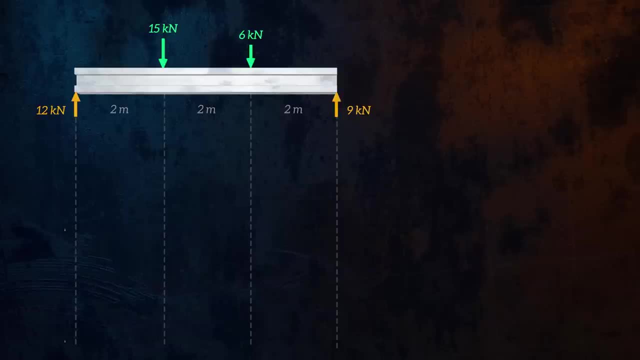 Now that all of the external loads acting on the beam are defined, we can draw the shear force and bending moment diagrams. We will start from the left-hand side of the beam. Let's draw the free-body diagram. Let's draw the free-body diagram for a location immediately to the right of the 12 kN reaction force. 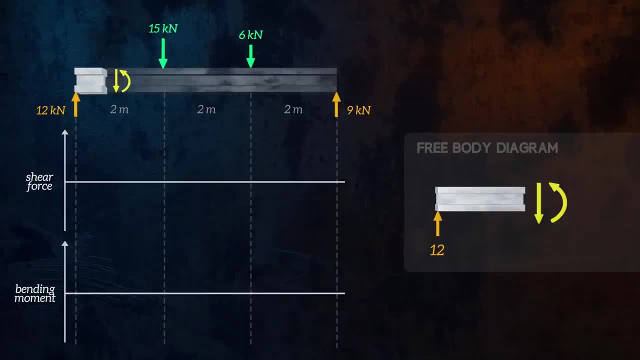 To maintain equilibrium, the shear force must be equal to the reaction force. We can draw this on our shear force diagram. The shear force will be constant until we reach the next applied force. The bending moment must be equal to the 12 kN reaction force multiplied by the distance x to the reaction force. 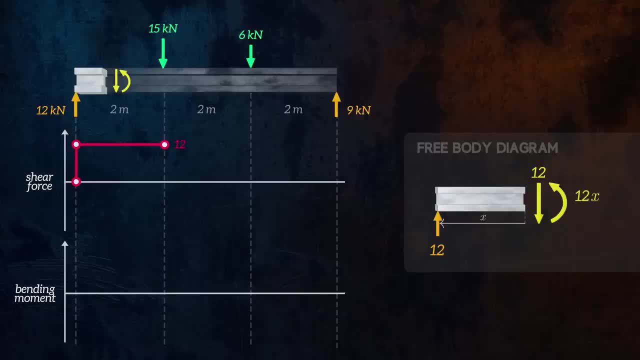 This gives us the equation for a straight line which we can draw on our bending moment diagram. We then repeat the process by moving the location of our cut further to the right. This time we place the cut immediately after the 15 kN force. 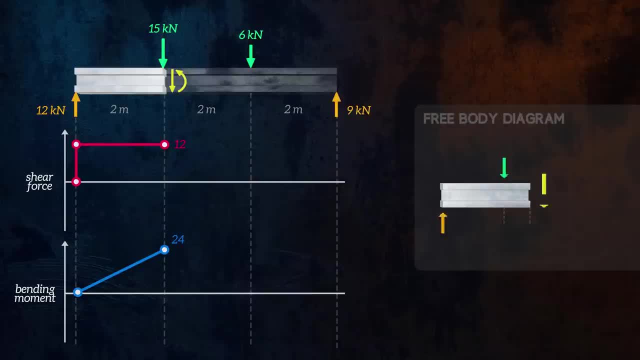 and we draw the free-body diagram again to determine the shear force and the bending moment. We repeat this process until we have covered the full length of the beam. We end up with the complete shear force and bending moment diagrams for the beam. We can now draw the shear force diagram for a dedicated beam. 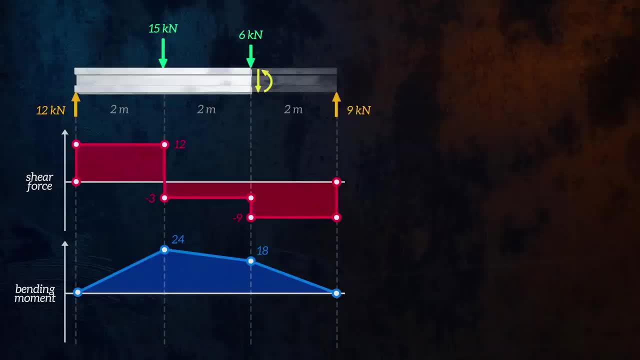 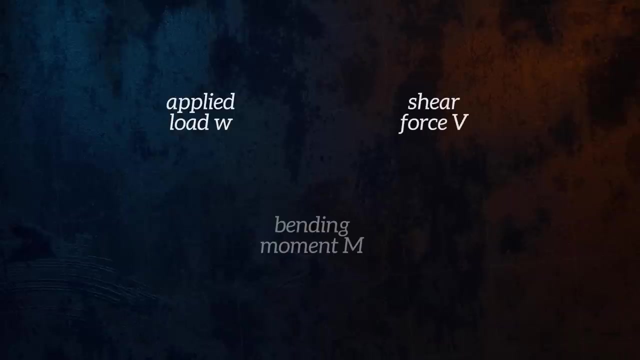 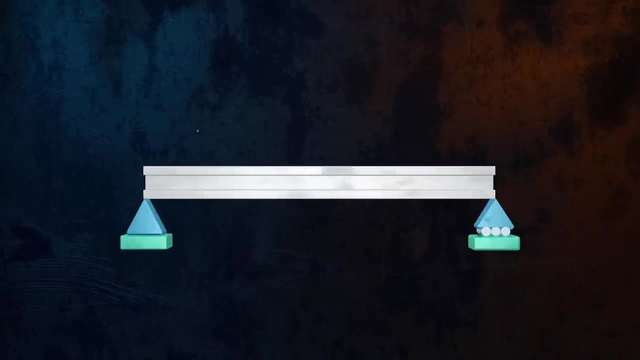 that example was a fairly simple one. for cases with more complex loading, drawing the shear force and bending moment diagrams can be more difficult. there are relationships between the applied loads, shear forces and bending moments which will help us better understand what our diagram should look like. let's consider a beam loaded by an arbitrary distributed force. we can 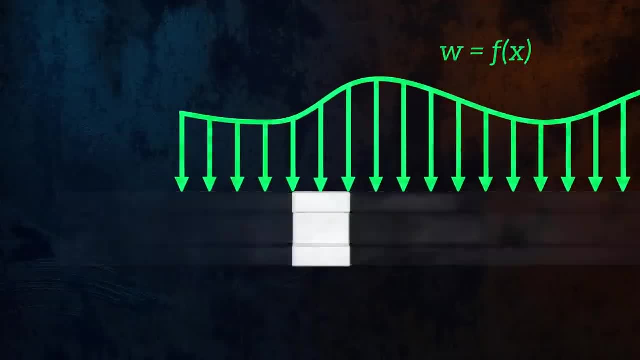 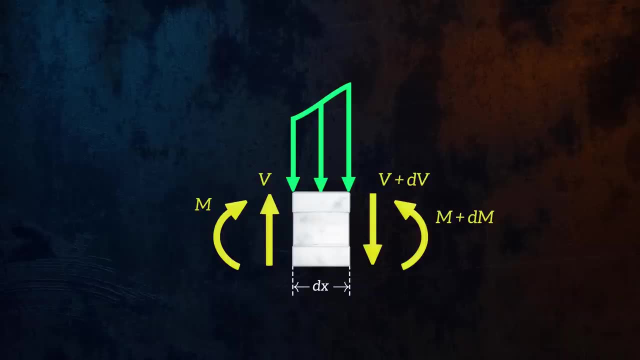 zoom in to look at an infinitesimally small segment of the beam with a width equal to DX, and draw the free body diagram over such a short section of the beam. the distributed force can be assumed to be uniform and we can replace it with an equivalent concentrated force by applying the 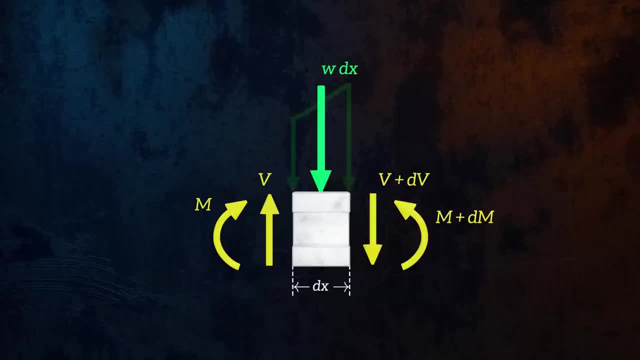 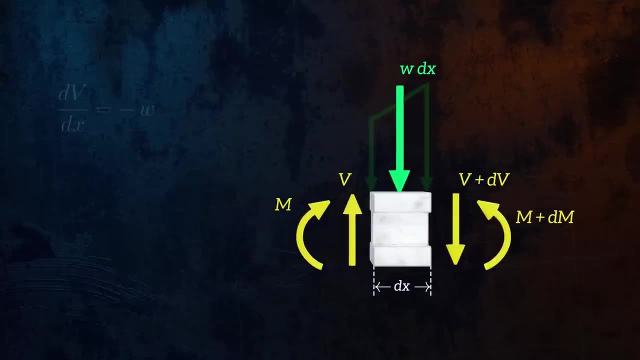 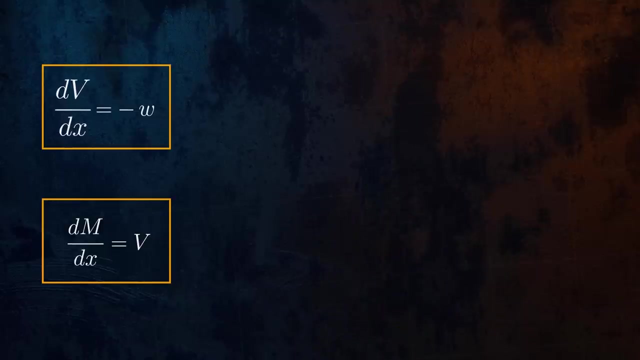 equilibrium equations to this free body diagram, it is possible to demonstrate that the following relationships exist between the applied distributed force, the shear force graph and the bending moment diagram and the distributed force graph: the shear force graph and the bending moment graph: the quantity DV over DX is the slope of the shear force curve and at a given point, 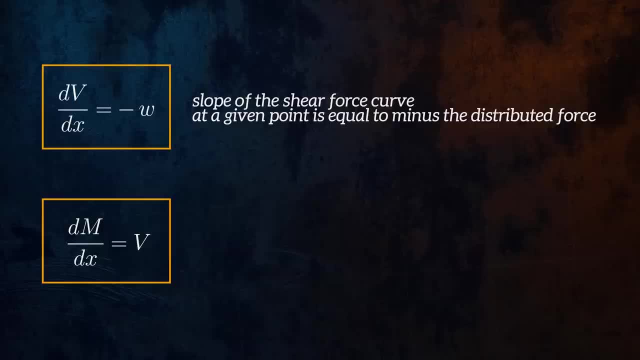 along the beam it is equal to minus the distributed force. similarly, DM over DX is the slope of the bending moment curve and at a given point is equal to the shear force. if we integrate the first equation, we can show that the change in shear force between two points 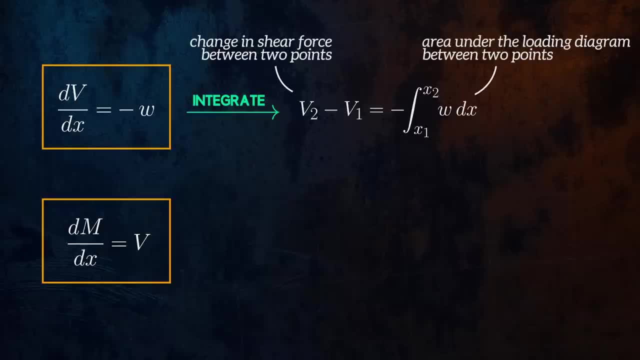 is equal to the area under the loading diagram between those two points. and if we integrate the second equation, we can show that the change in bending moment between two points is equal to the area under the shear force curve. this is really useful information we can use to help construct. 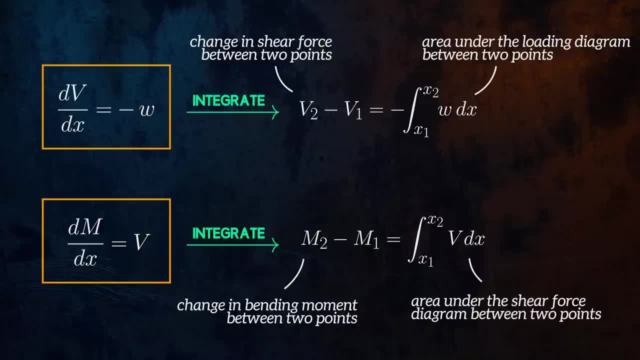 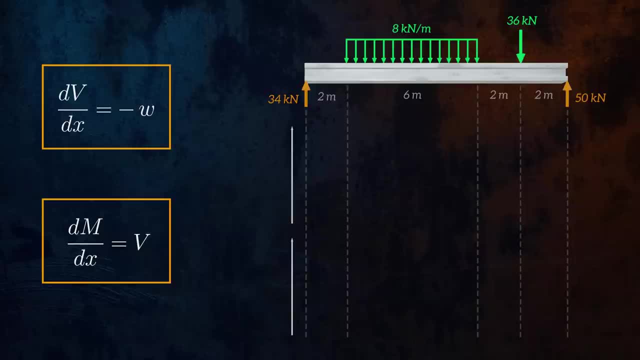 or sense, check our shear force and bending moment diagrams. let's take a look at an example. this beam has an applied distributed force in a concentrated force. let's quickly draw the shear force diagram by using the free body diagram method. we can show that the bending moment curve for the section of 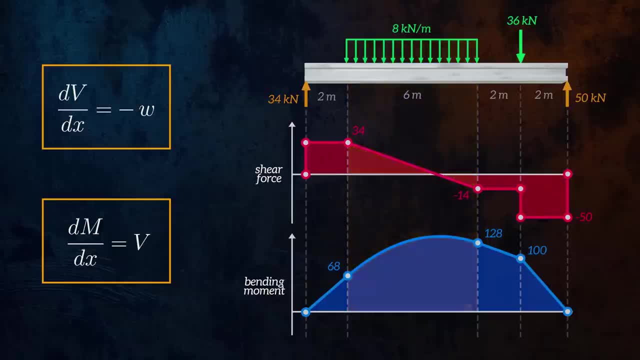 the beam under the distributed force is defined by the quadratic equation negative 4x squared plus 34x plus 68. if we differentiate this equation we get negative 8x plus 34 which, based on the D m over DX equation above, we now know is the equation for the shear force curve in this. 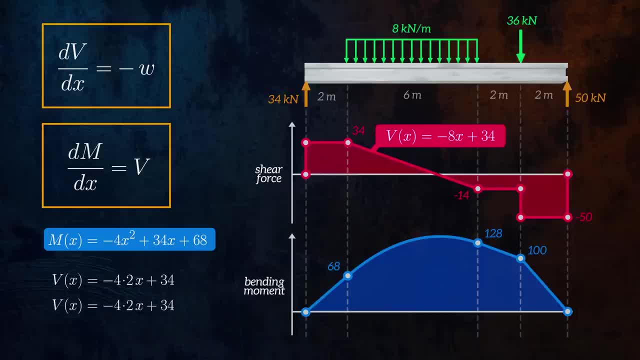 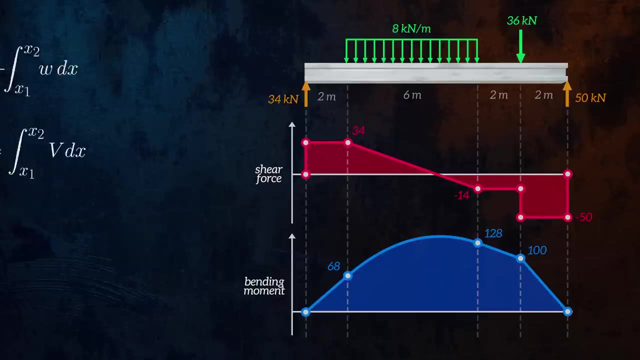 section of the beam. if we differentiate again, we get negative 8, which is the equation for the distributed force. this is a great way to sense check your shear force and bending moment diagrams. another way of checking your diagrams is using the area equations I mentioned earlier. the area under the shear force curve highlighted here is equal to the shear force curve squared plus. 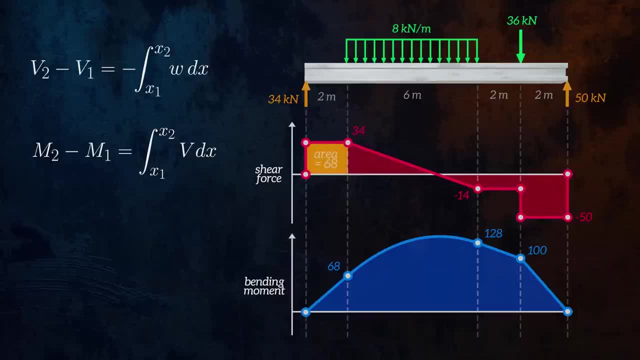 to 34 times 2, which is 68.. This is equal to the change in bending moment over this section of the beam. We can also calculate the area under the shear force diagram for the beam section. under the distributed force, The total area of this section is equal to 72.3 minus 12.3, which is 60.. 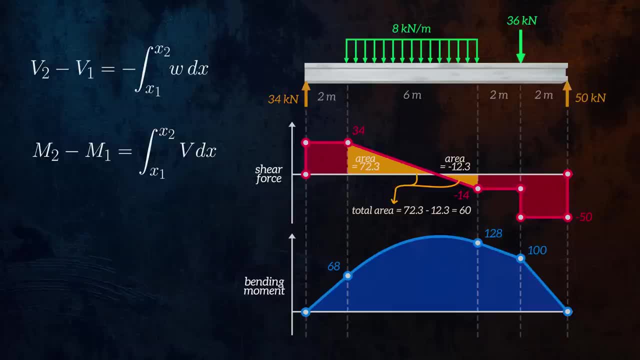 This is equal to the change in bending moment of 60 kilonewton meters over this section of the beam. Where concentrated forces are applied, there is a sudden jump in the shear force diagram, And where concentrated moments are applied, there is a sudden jump in the bending moment diagram. 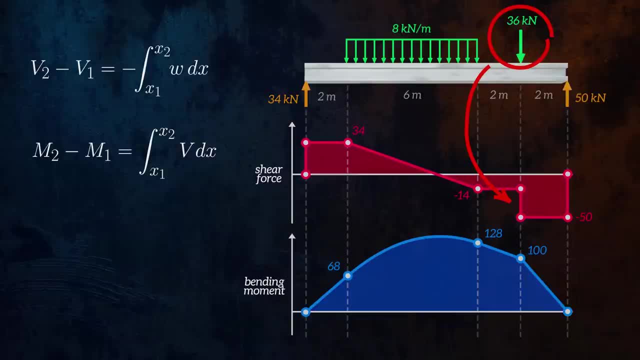 These equations will not be applicable across discontinuities in the diagrams. One final observation we can make based on these equations is that when the shear force is equal to zero, the bending moment curve will be at a local minimum or maximum. Let's look at one last example. 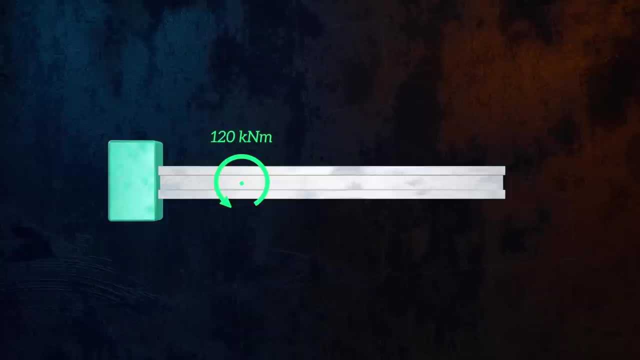 Here we have a cantilever with an applied concentrated moment of 120 kilonewton meters and a distributed force of 6 kilonewtons per meter. Again, we start by drawing the free body diagram, Because the support is fully fixed. we have vertical and horizontal reaction forces. 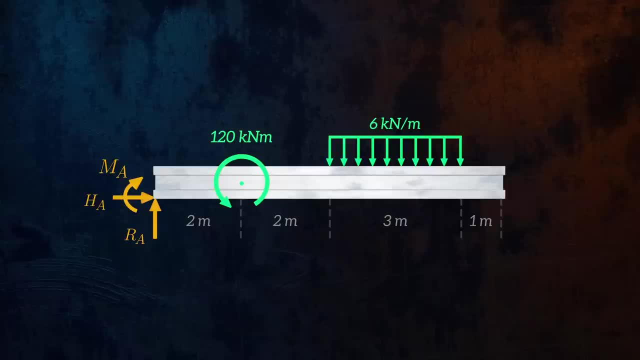 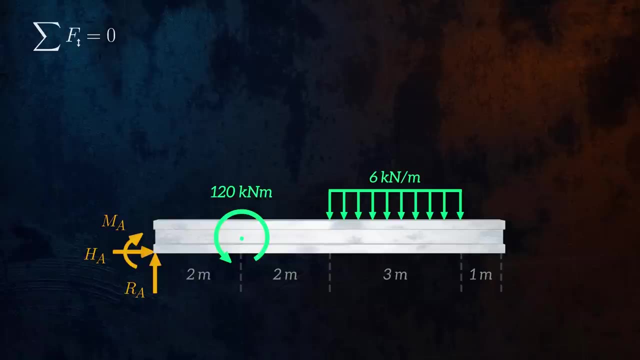 Ra and Ha and reaction moment Ma. Let's look at our first equilibrium equation. The sum of forces in the vertical direction is equal to zero. In this case, the only forces acting in the vertical direction are the reaction force, Ra, and the distributed force. So Ra is equal to 6 times 3, which is 18.. 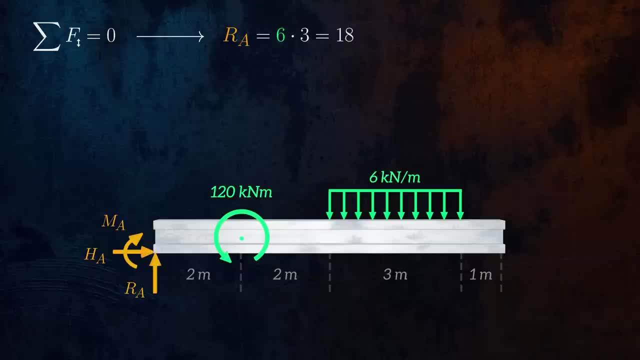 Ha is the only force in the horizontal direction, so it must be equal to zero. Next, we can take the sum of the moments acting at point A. Let's look at our first equilibrium equation: The sum of forces in the vertical direction is equal to zero. 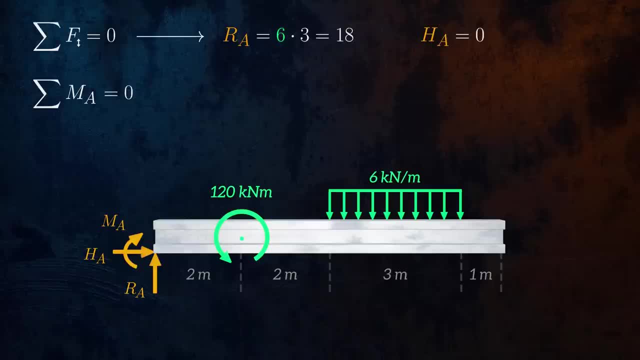 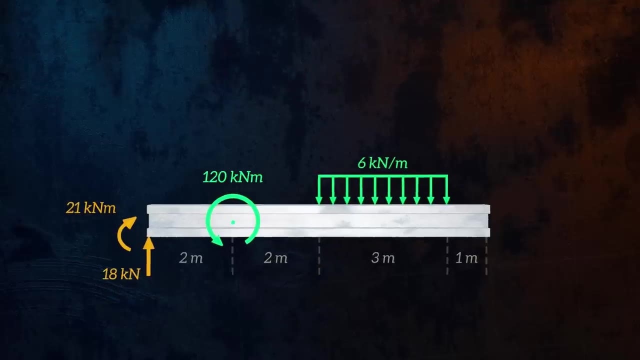 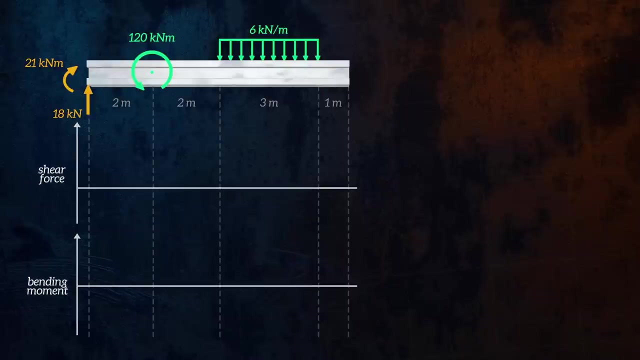 In calculating the moment caused by a uniformly distributed force, you can remember that it is equal to a concentrated force located in the middle point of the load. This gives us Ma equals 21.. To calculate our shear forces and bending moments, we will start on the left side of the beam and move towards the right. 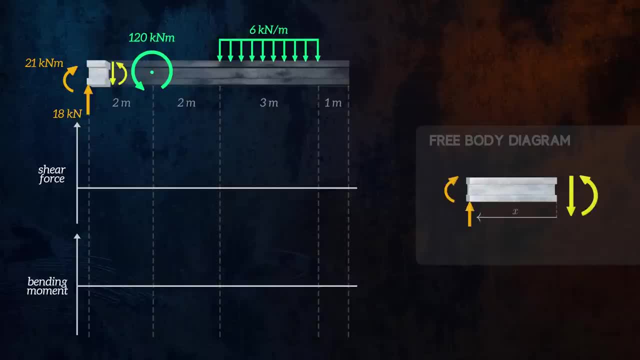 This is our first free body diagram. The shear force calculation is easy, as we only need to consider the reaction force of 18 kN. The bending moment needs to take into account the reaction moment and the reaction force At x equals zero. the bending moment is equal to the reaction moment of 21 kN meters. 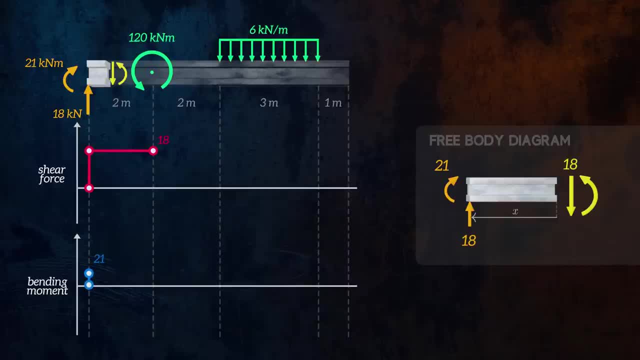 As we move to the right, we also need to consider the moment caused by the 18 kN reaction force. This gives us Ma equals zero. This gives us the equation for a straight line. We can then move our cut to the right of the concentrated moment. 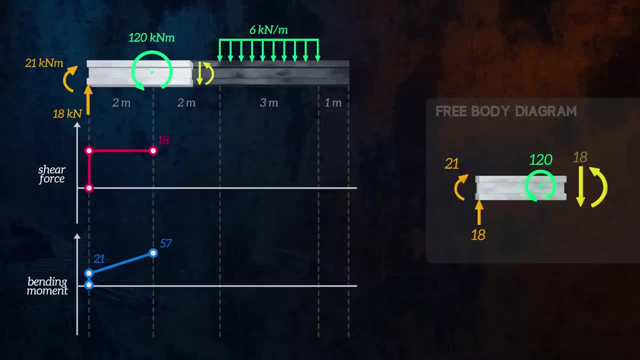 The moment won't affect the shear force, which will remain constant at 18 kN until we reach the distributed force, But it does cause the bending moment to suddenly drop by 120 kN meters. After the drop, the bending moment is again defined by a straight line.